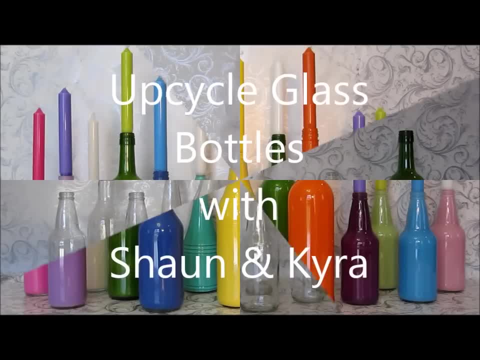 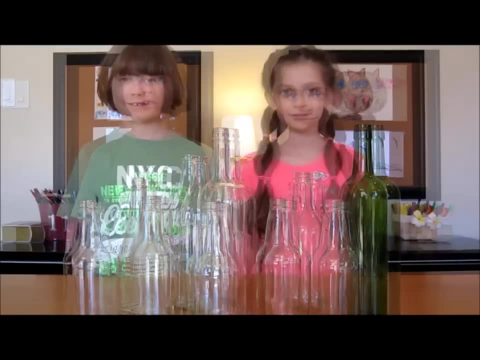 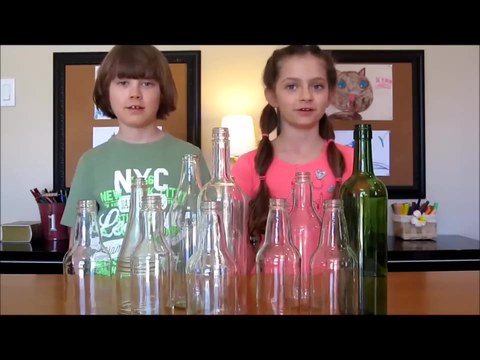 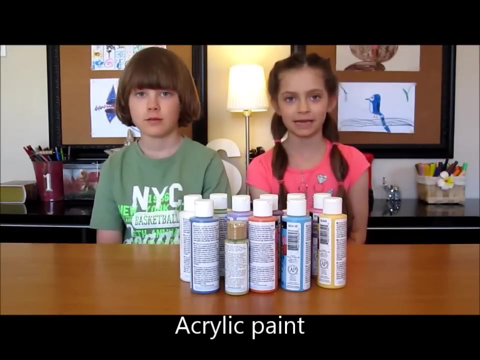 Hello everybody, and today we are going to upcycle glass bottles. You can use all kinds of bottles: Wine bottles, beer bottles, oil bottles, vinegar bottles, soya bottles and water bottles. You will also need acrylic paint in any color you like. Protect your. 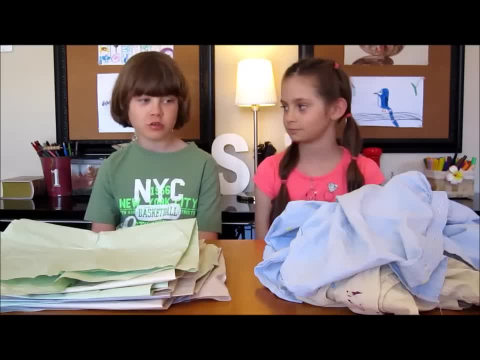 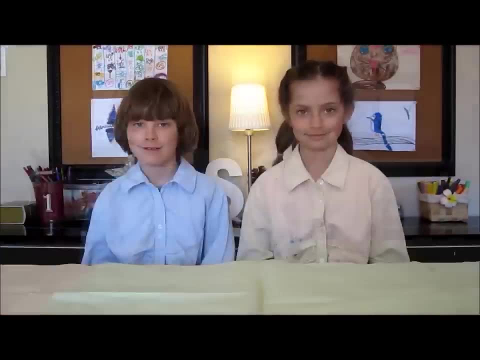 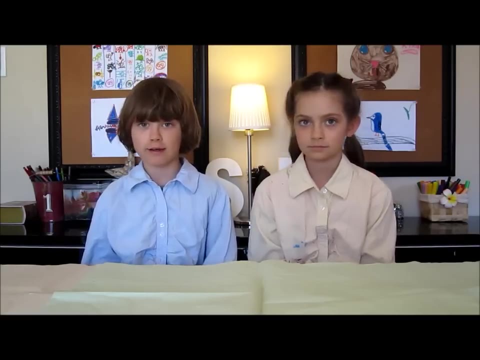 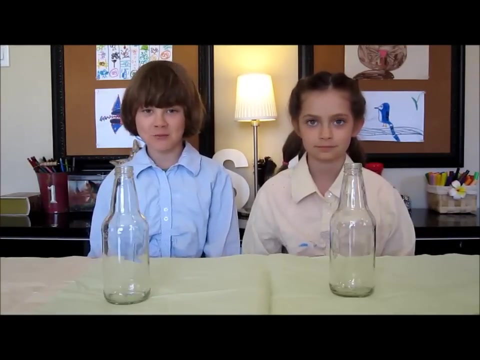 table with old paper and protect your clothes with paint clothes. Keep in mind that acrylic paint is permanent and waterproof when it's dried, Always have a wet towel in hand to clean the paint, if needed. First, you will need to prepare your bottles. Let the bottles 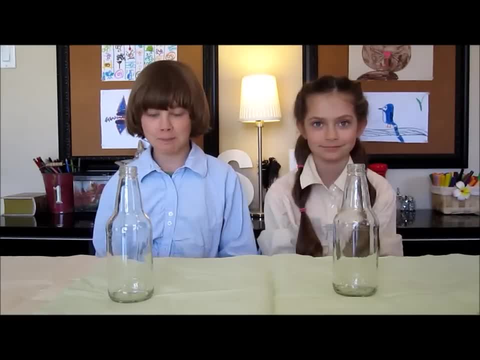 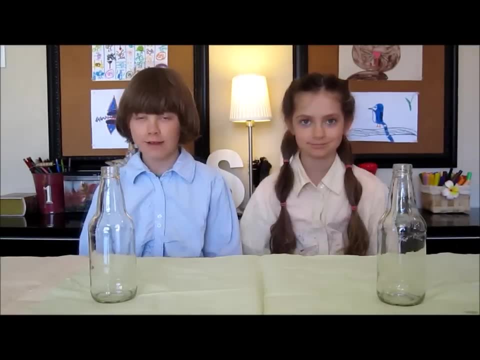 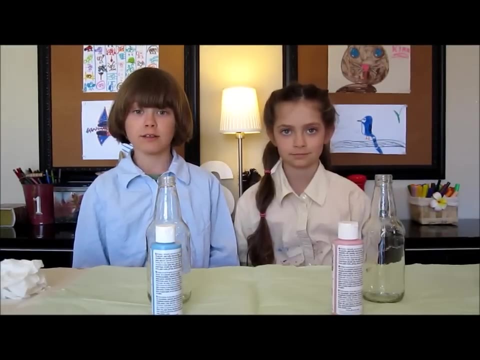 soak in soapy water for a few hours, Then peel off the sticker If there is still some glue residue. use a sticker cleaner that you find at the store And wash your bottles carefully and let it dry completely. When your bottles are clean and dry, this is what you do. Take the acrylic paint and pour a. 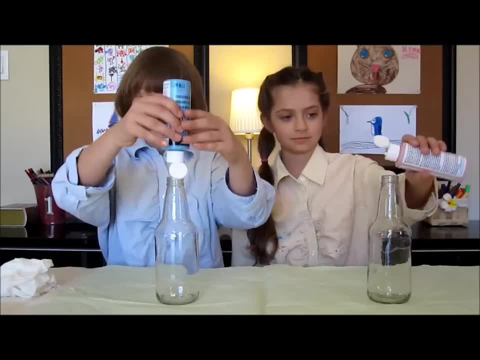 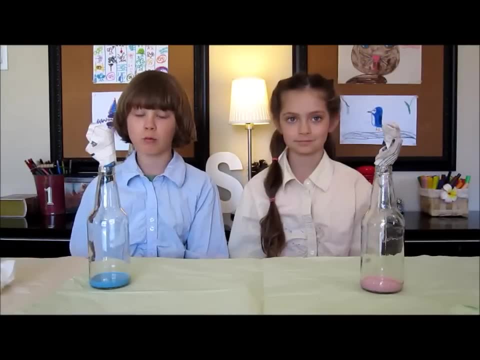 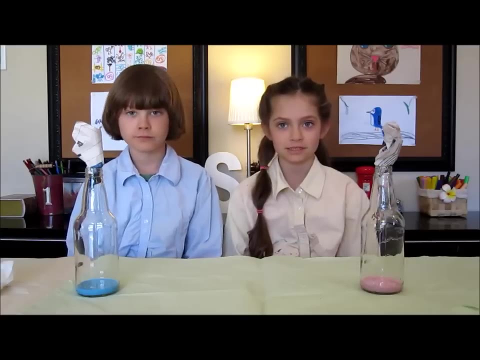 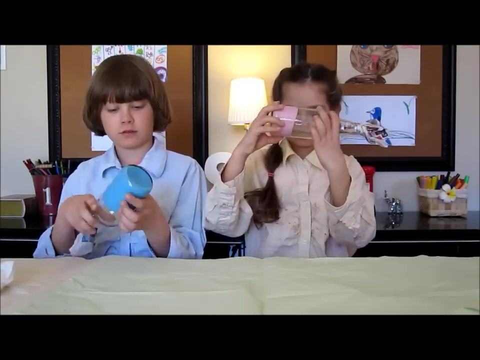 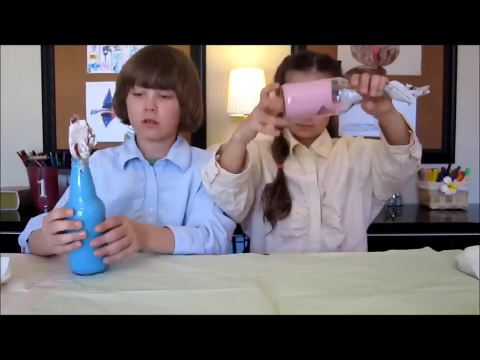 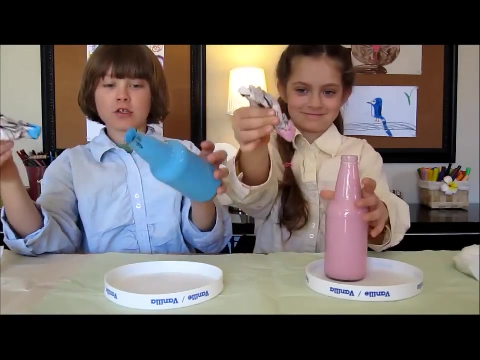 good quantity inside the bottle. Close the opening with old paper. Now take your bottle and turn it around so the paint covers all the inside of the bottle. When you are done, take out the newspaper and turn it over to let the extra paint dry. 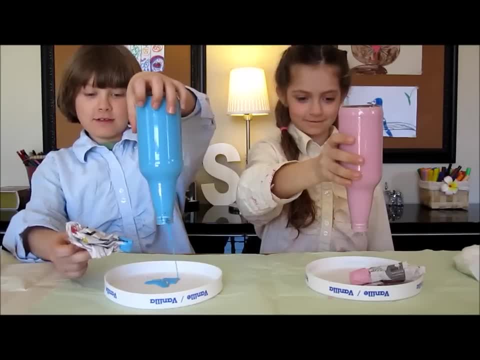 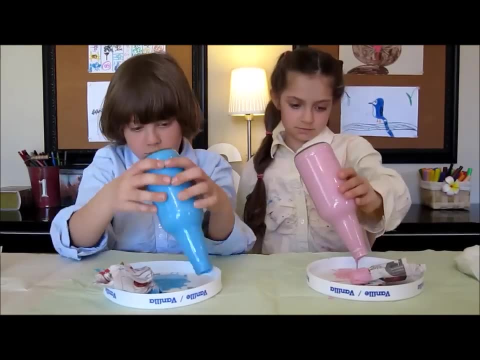 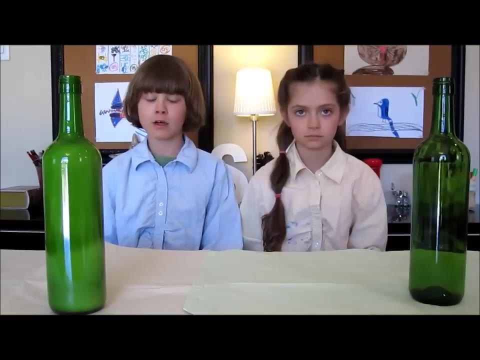 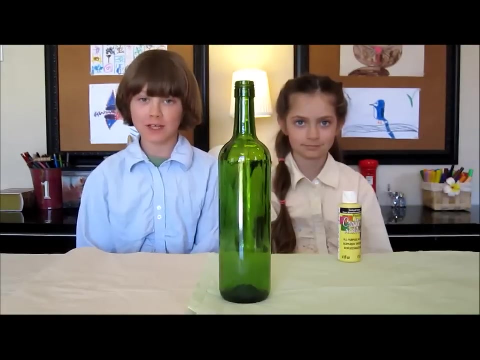 When you are done, take out the newspaper and turn it over to let the extra paint dry come out. it could take two or three days to dry. you can also use colored glass bottles. for this one we use the white paint. we're going to try a yellow paint. 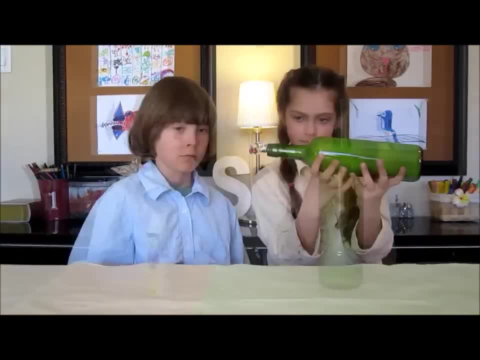 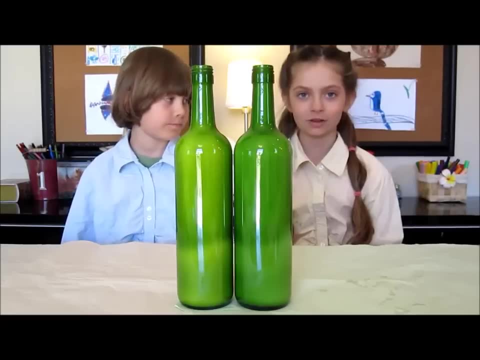 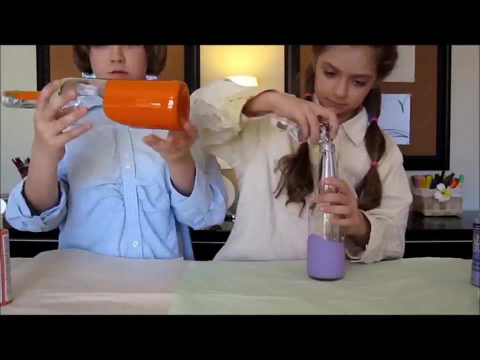 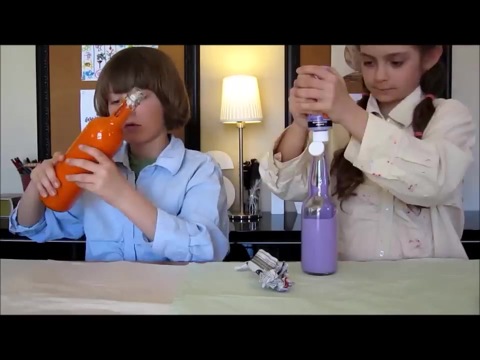 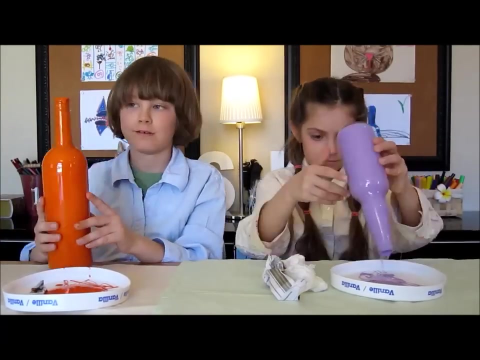 now the yellow and white one kind of looks the same. thanks for watching and we'll see you next time. bye. 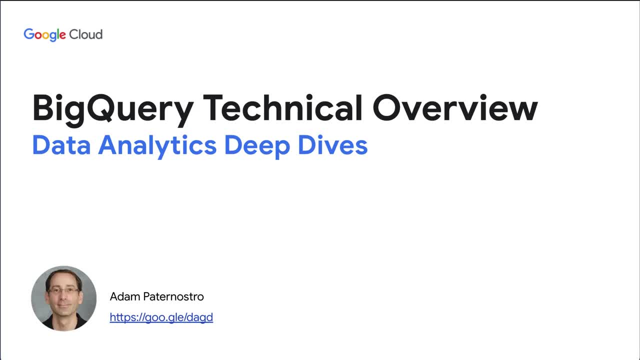 Hello everyone, Welcome to the BigQuery technical overview. We will take a tour of BigQuery, from data ingestion, streaming data governance, along with data quality machine learning, all the way through our intelligent serverless infrastructure. So let's get started. 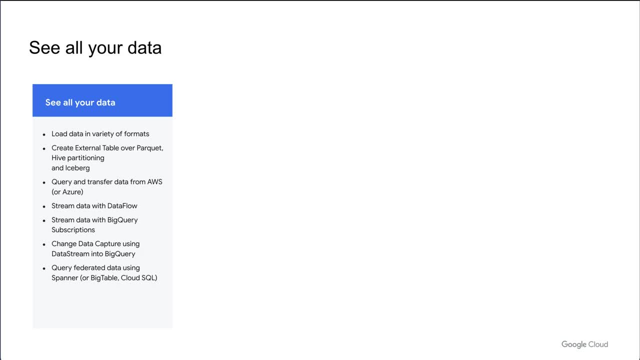 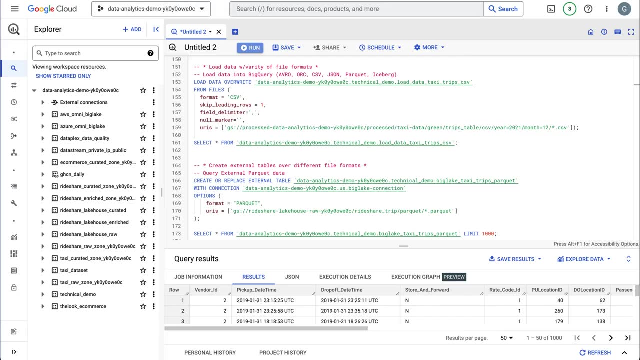 The first thing I'd like to show is how customers can see all their data. Data lives everywhere, and BigQuery can bring all your data together and process it at scale. So let's head over to BigQuery and see how this works. So I'm in BigQuery now, And the first thing I'd like to 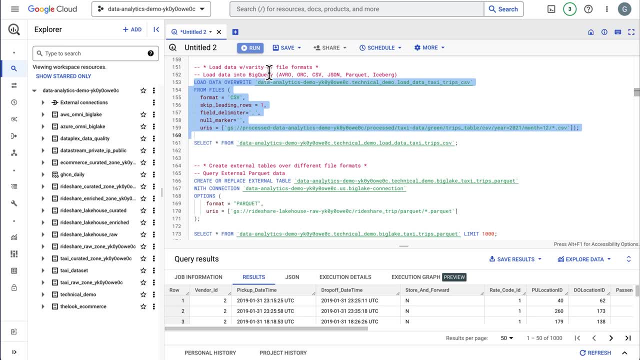 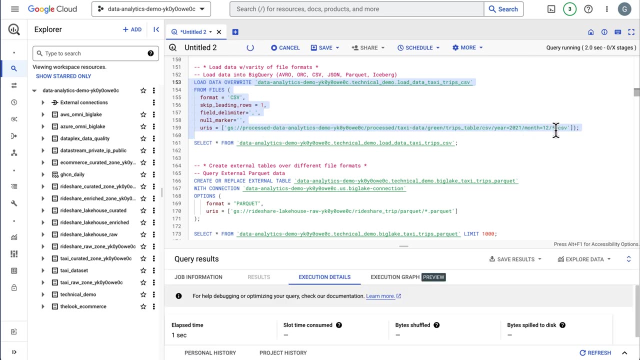 show is how we can ingest data into BigQuery. So this is a load command done in SQL And we support all the popular formats up here- Avro, Ork, JSON, Parquet, Iceberg- And we are bringing in a CSV file, in this case from our Google Cloud Storage account, So very easy to use. 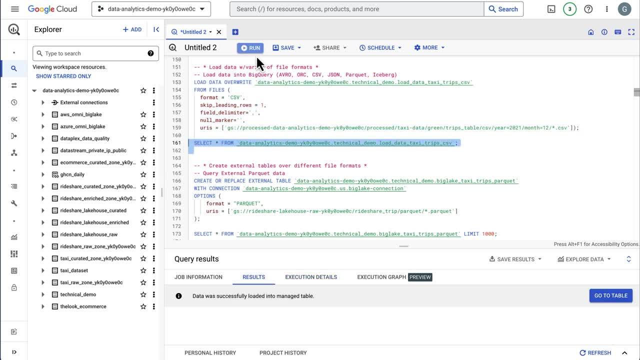 And you can do this through our CLI, directly through SQL or SDKs. We support also third-party ETL tools. So after we've run this command, we can see we've ingested the data down here And it's available immediately in BigQuery. So the next piece is creating: 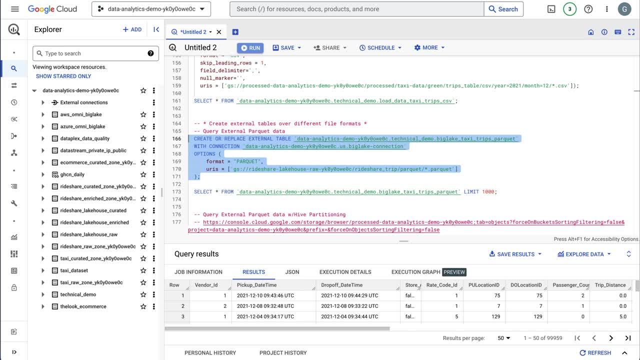 external tables. So a lot of customers want to support querying their data on their data lake directly in place if you have a data mesh or a lake house architecture, So it's important that we can query the data directly on storage And in this case we're creating an external table.